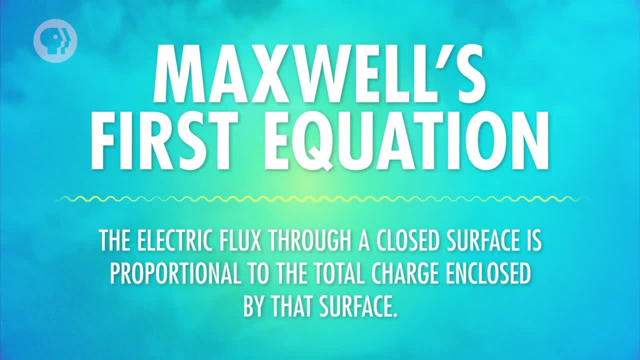 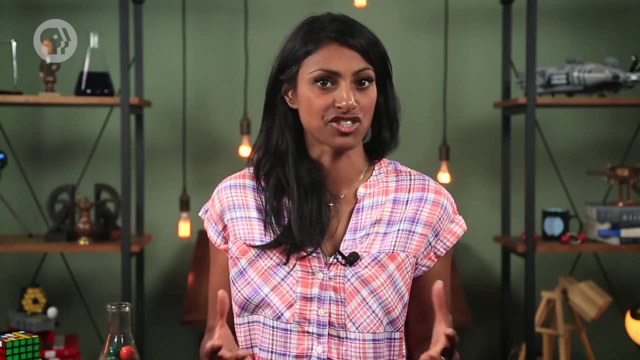 Maxwell's first equation is a form of Gauss's law, which states that the electric flux through a closed surface is proportional to the flow of electric current And it's proportional to the total charge enclosed by that surface. A closed surface in this case is just the surface of any shape that completely encloses a charge, like a sphere or any other three-dimensional shape. 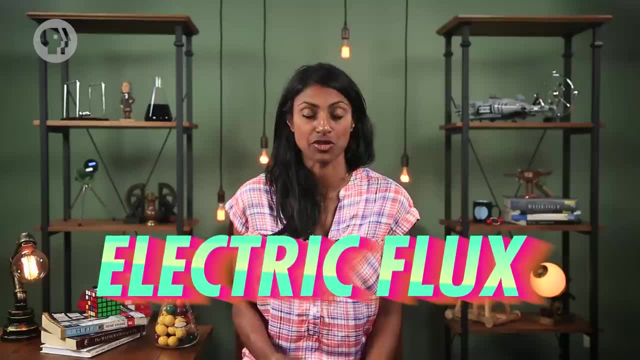 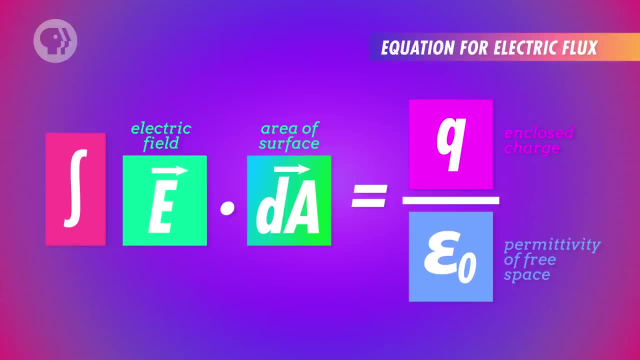 And electric flux is a measure of the electric field that passes through a given area. Mathematically, this equation says that electric flux is the integral of the electric field over the area of the surface, which is equal to the enclosed charge divided by the permittivity of free space. 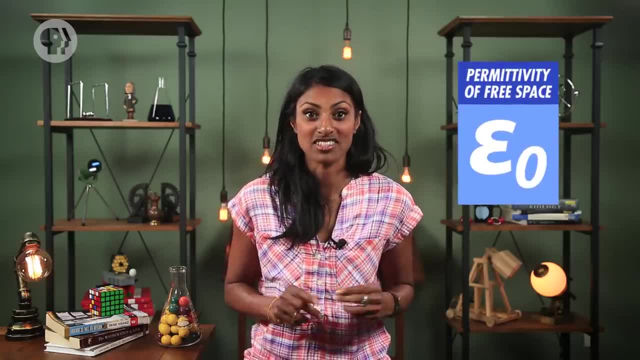 I won't blame you if you don't remember, but the permittivity of free space is a constant of proportionality that we've used. So what does that mean? It's a constant of proportionality that we've used before. that relates electric charge to the physical effect of electric fields. 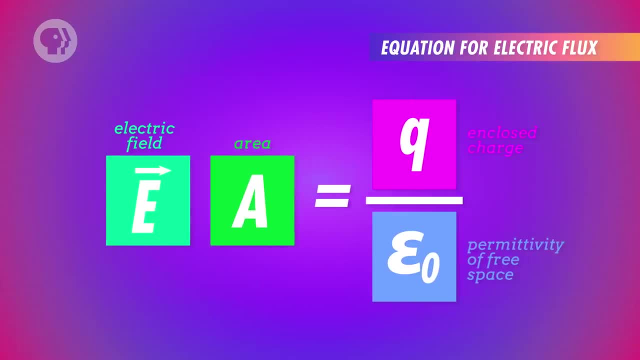 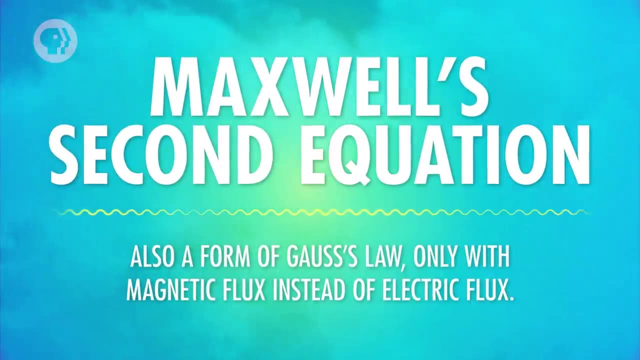 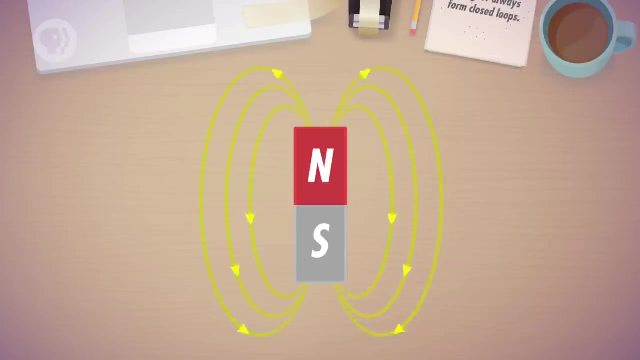 If the electric field is a constant over the surface, then the left side of the equation becomes E times A. Maxwell's second equation is also a form of Gauss's law, only with magnetic flux instead of electric flux. Magnetic sources are always dipoles, with a north and south pole and magnetic field lines that leave from the north pole and return back to the south. 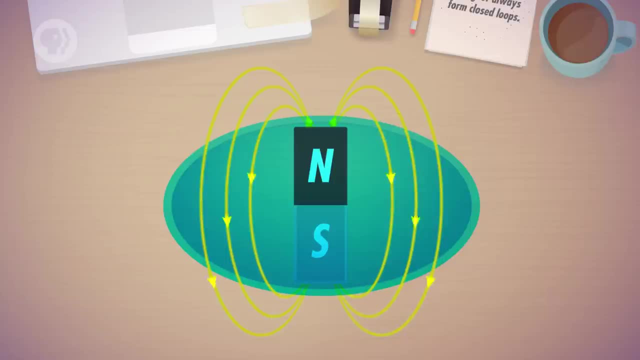 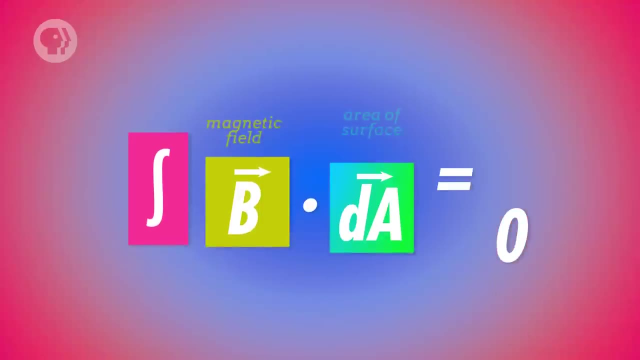 When you're looking at how a magnetic field interacts with the surrounding surface, you see that the field lines that leave the surface out of the north pole must enter back through the surface to reach the south pole. This results in the overall magnetic flux being zero. 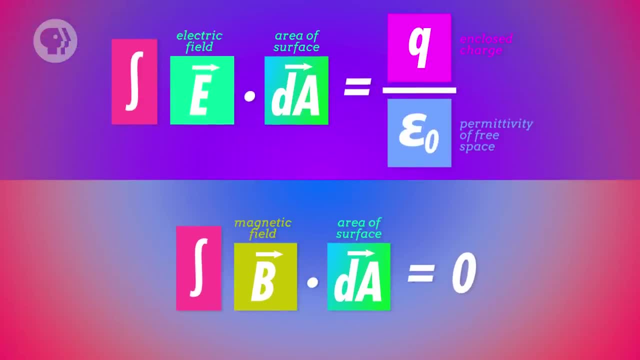 If you compare this with Maxwell's first equation, you can tell that the format with the integral of the magnetic field over the surface area is the same, but here the integral will always equal zero for a closed surface. Now Maxwell's third equation doesn't have anything to do with Gauss's law. 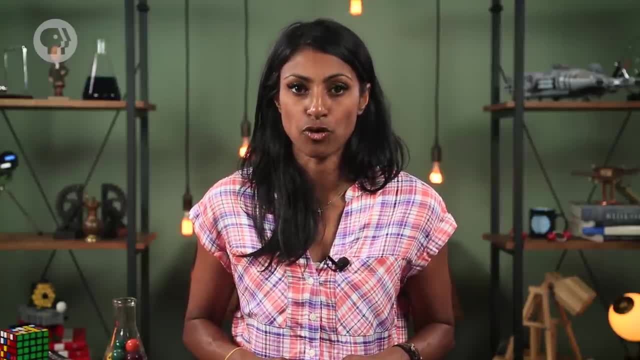 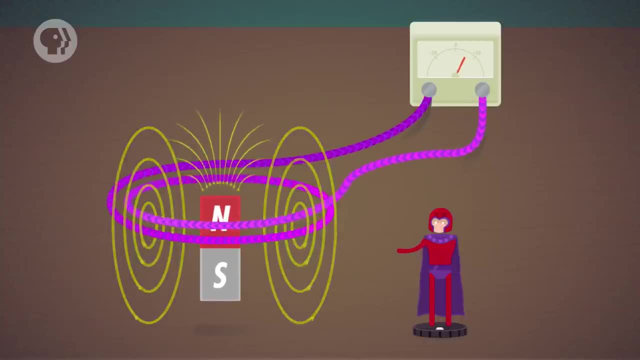 Instead, it's Faraday's law, but slightly different than how we've seen it before. This is how we've seen it before. If you remember, Faraday's law of induction says that a changing magnetic field will induce an electromotive force in a loop of wire. 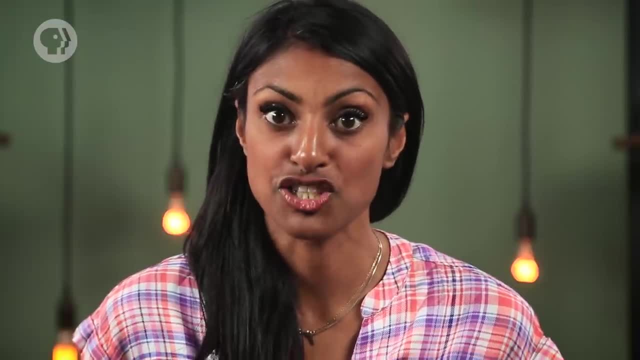 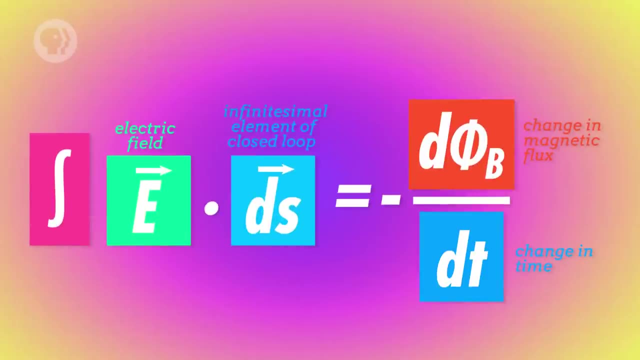 Maxwell's version is more general, simplifying Faraday's law to show the value of that induced EMF. It says that the EMF is equal to the line integral of the electric field over a closed loop. So with this equation you can see the connection between a changing magnetic flux and an induced electric field. 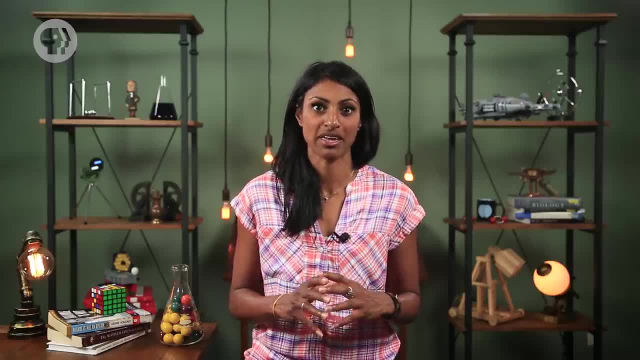 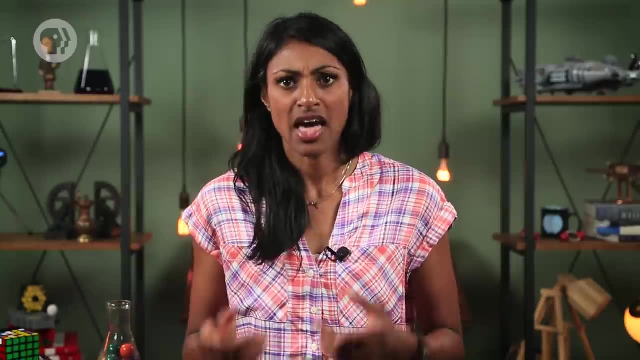 The fourth and final equation is one that Maxwell made the most tweaks to in order to make it applicable to all electromagnetic phenomena. Maxwell's first and second equations were so similar- one for electric fields and one for magnetic fields- that he knew there must be an equation that complemented Faraday's law as well. 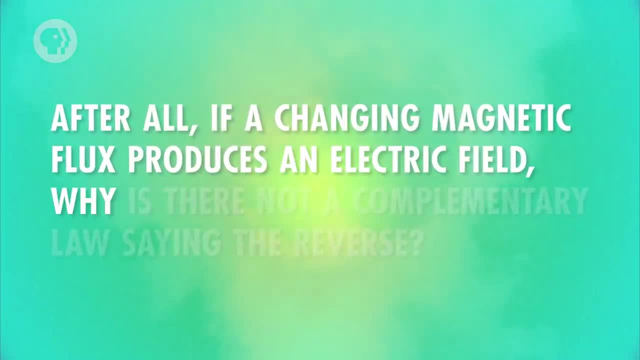 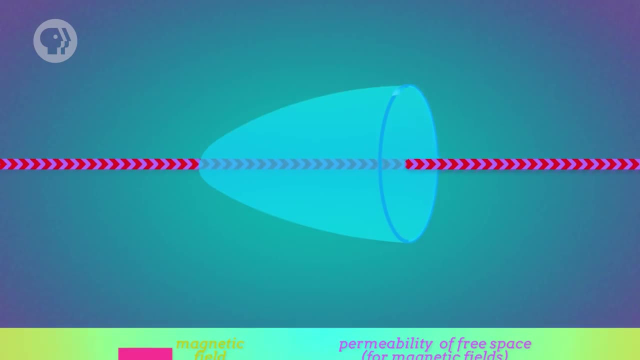 After all, if a changing magnetic flux produces an electric field, why is there not a complementary law saying the reverse? Why couldn't a changing electric flux result in an induced magnetic field? Here Maxwell started with Ampere's law, which states that a current through a wire induces a magnetic field around a path surrounding the wire. 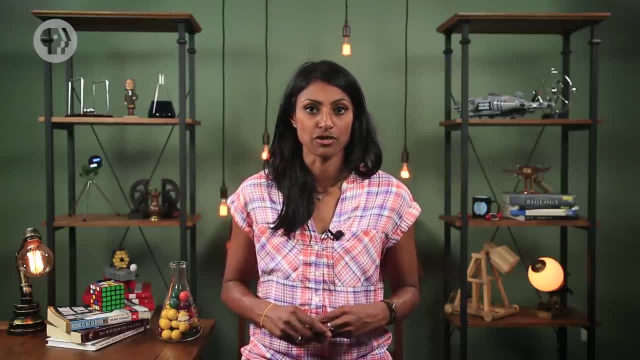 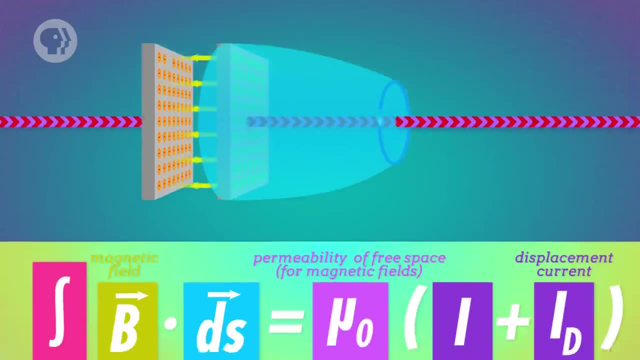 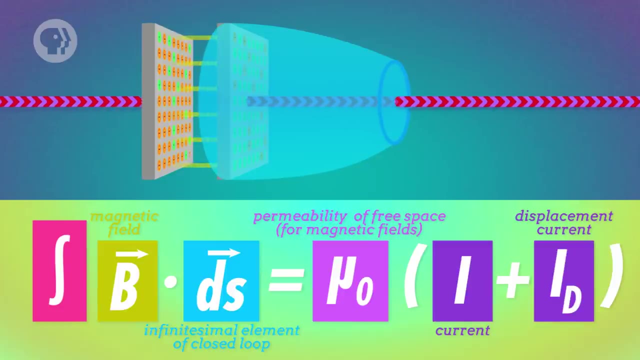 In order to make this equation work for all possible electromagnetic scenarios, Maxwell needed to consider a situation where a magnetic field is induced, but not from the flow of current Picture a charged capacitor that's connected to wires on both sides. As the capacitor discharges, current runs through both wires, generating a changing magnetic flux, just like Ampere's law says. 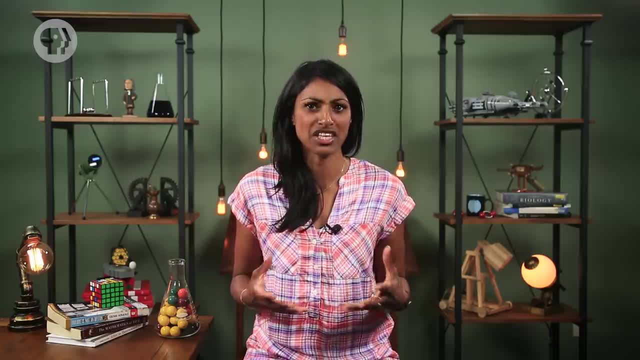 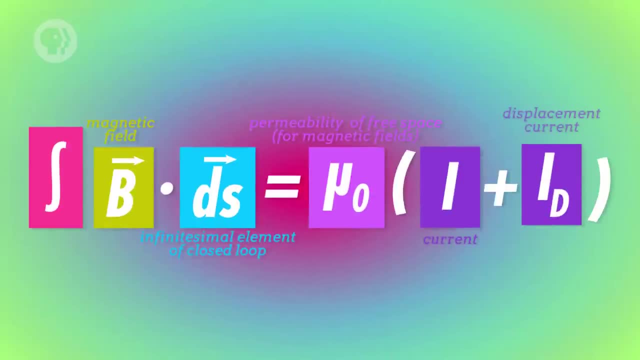 But a changing magnetic flux is also induced between the two plates. when there's no wire connecting the plates, However, there is a changing electric field and it acts like a wireless current. In order to account for the magnetic flux generated by this wireless current, 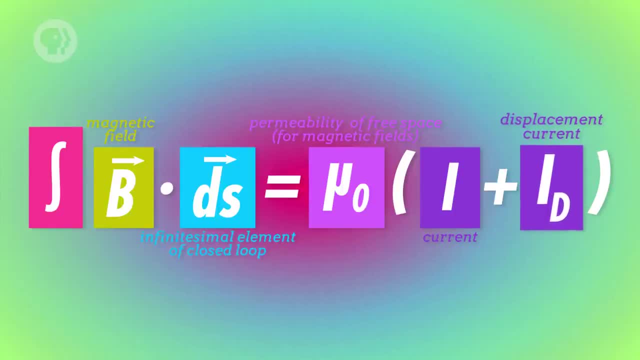 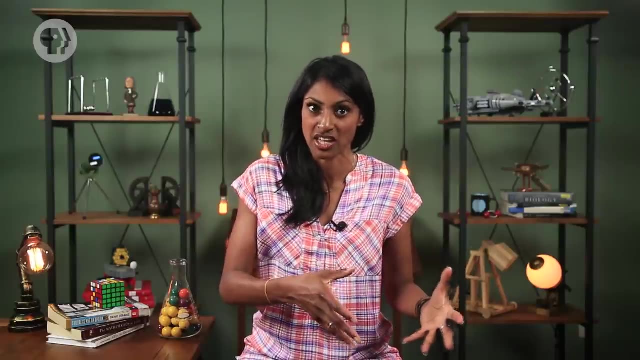 Maxwell added what's known as the displacement current into Ampere's law to complete the equation. Despite being called the displacement current, it isn't really an electric current. It's just called that because it fits into the equation just like an actual current does. 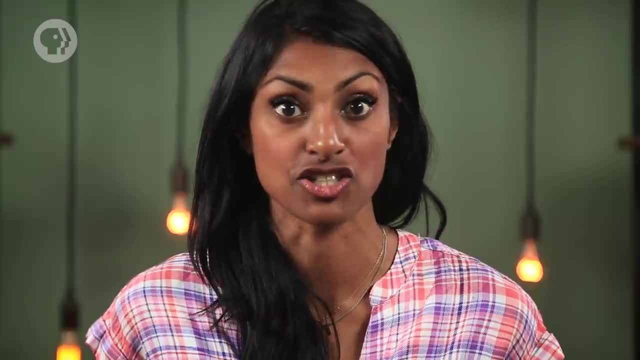 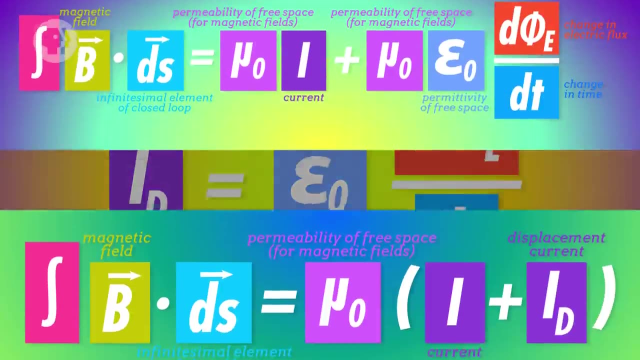 Mathematically, the displacement current is equal to the change in the capacitor's charge over time, And that is equal to the change in electric flux over time, multiplied by the permittivity of free space constant. With the addition he made to Ampere's law, Maxwell's equations were complete. 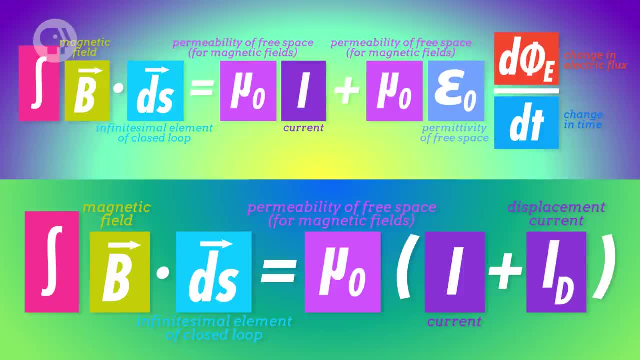 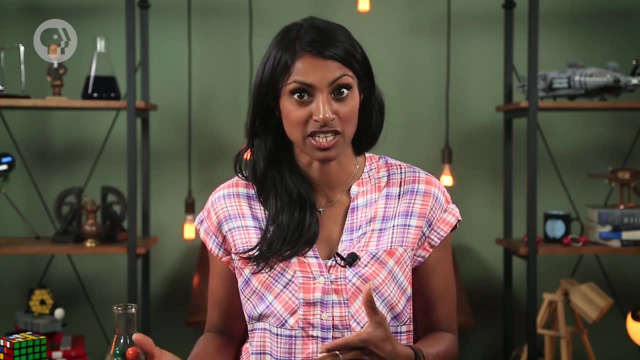 And using his laws. today we can see a pattern in the production of electric and magnetic fields. If a changing electric field is generated, then a magnetic field is induced, which results in a changing magnetic field that induces an electric field, and the cycle continues. 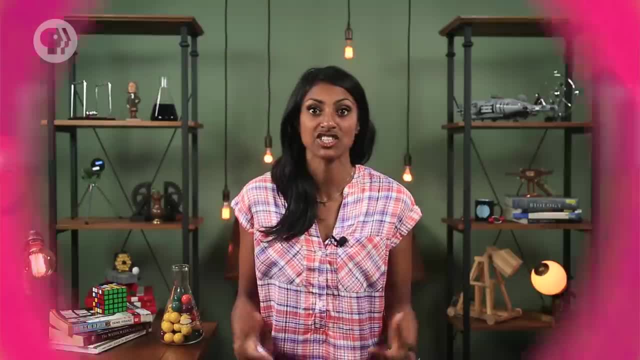 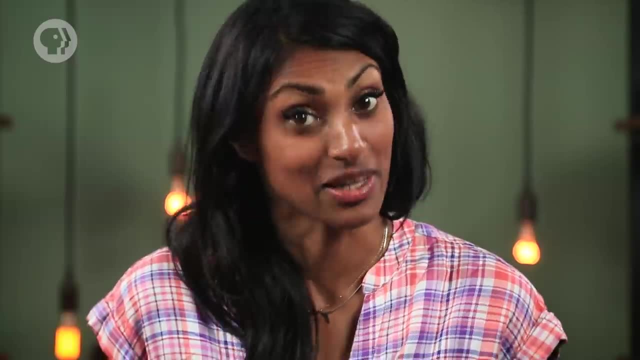 These oscillations are electromagnetic waves, and they're made up of changing electric and magnetic fields that travel through space. Maxwell believed that we could reproduce electromagnetic waves in the laboratory, and he was right To prove it. let's look at an object that can produce electromagnetic waves and transmit them through the air – an antenna. 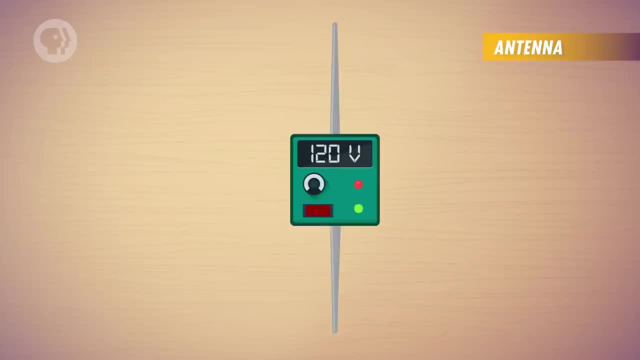 This antenna is made up of two conductive rods, each attached to opposite ends of an AC generator. When the antenna is operating, the two rods switch between being positively charged and negatively charged as the generator changes voltage. And when one rod is positively charged, the other is negatively charged, and vice versa. 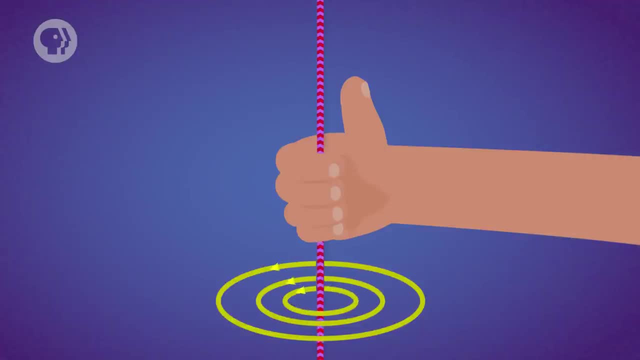 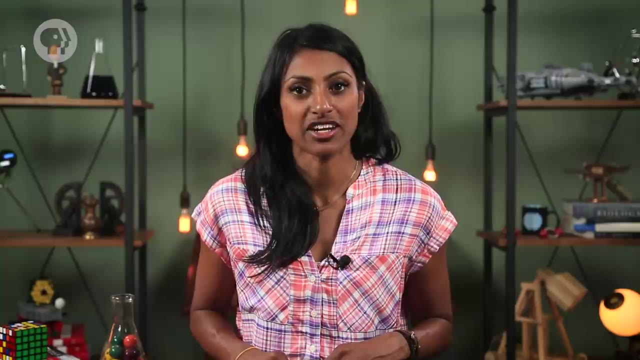 When electric current travels up into the top of the rod, you can use the right-hand rule, pointing your right thumb in the direction of the current, to see how the magnetic field flows around the antenna. The electric fields generated by the antenna itself are easier to track. 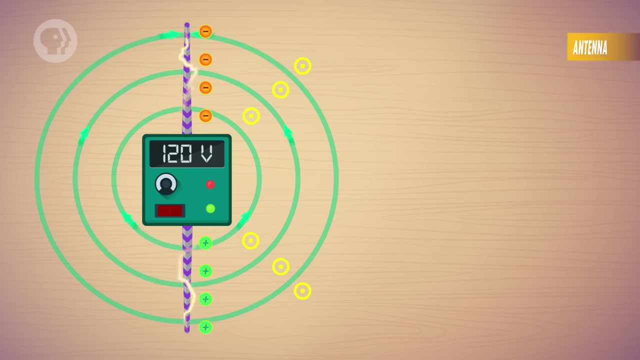 since they'll just go from the positive rod to the negative rod. But as the direction of current switches, the direction of both the electric and magnetic fields, change, And as the rods switch their charges, the waves generated by the initial charge distribution continue to propagate away from the antenna. 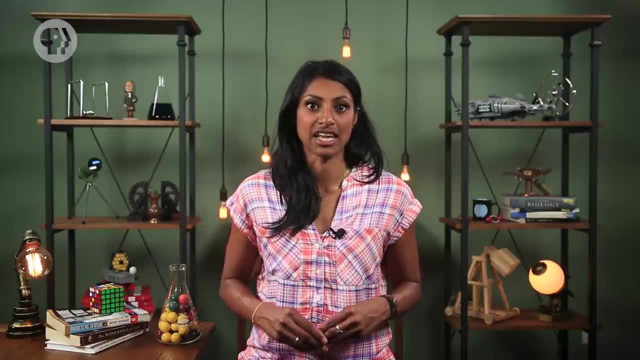 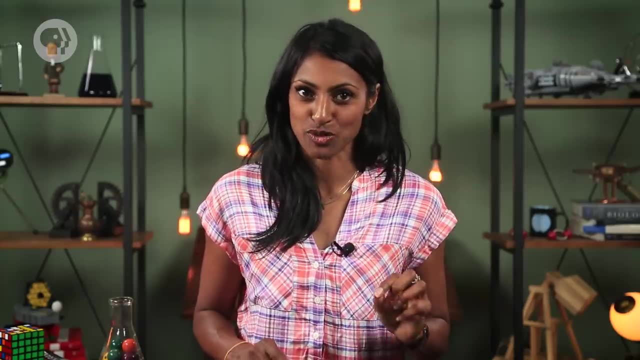 So if you were standing away from the antenna, you would be able to measure an electric field and magnetic field that are both constantly changing. Now what would that look like? To grasp the effect of changing fields of motion, let's model an electromagnetic wave as it travels through three-dimensional space. 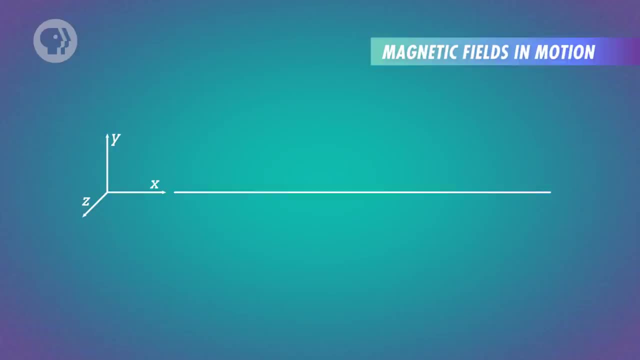 First note the direction that the wave is traveling in in the x-direction. Now plot the electric field oscillating back and forth in the y-direction. The electric and magnetic fields always act perpendicular to one another, so the magnetic field will oscillate in the z-direction. 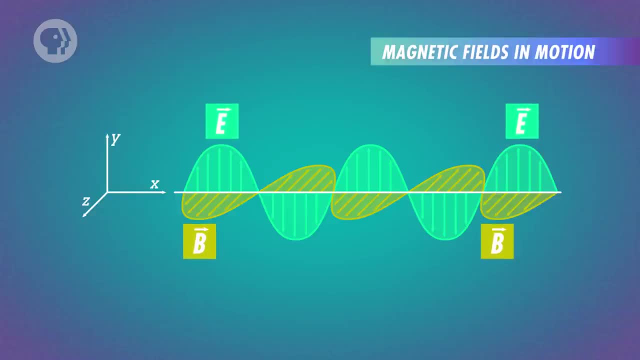 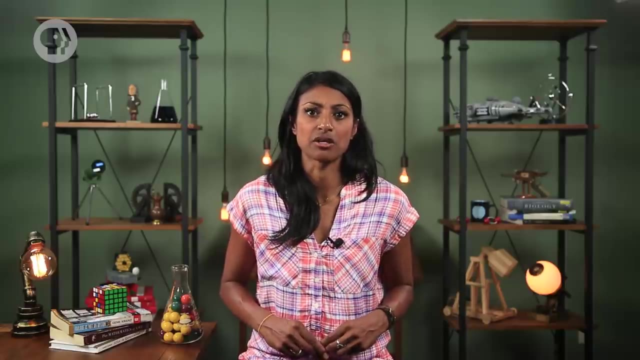 Note that the electric and magnetic fields both peak at the same time, so they're in phase. These electromagnetic waves are a type of transverse wave, which means both fields – electric and magnetic – act in directions that are perpendicular to the direction in which the wave is moving. 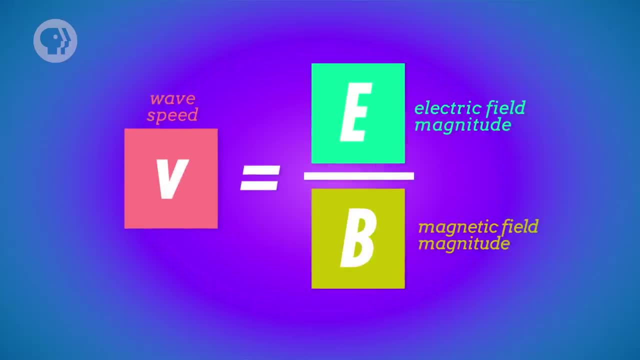 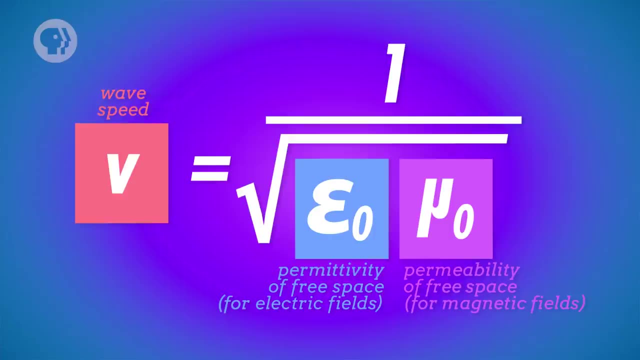 And how fast do these waves travel? Maxwell calculated that the speed of each wave is equal to the electric field's magnitude divided by the magnetic field's magnitude. This equation simplifies down to an equation. This equation simplifies down to an equation with two constants: the permittivity of free space for electric fields- epsilon-naught- and the permittivity of free space for magnetic fields- mu-naught. 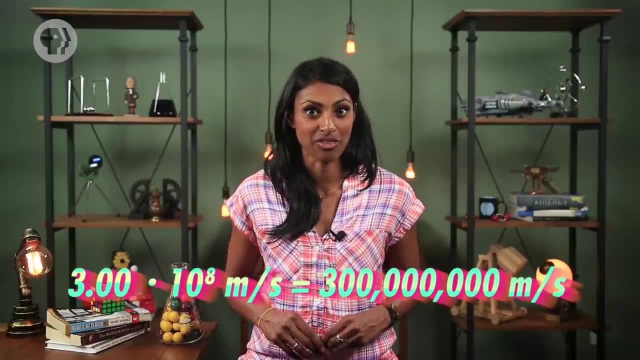 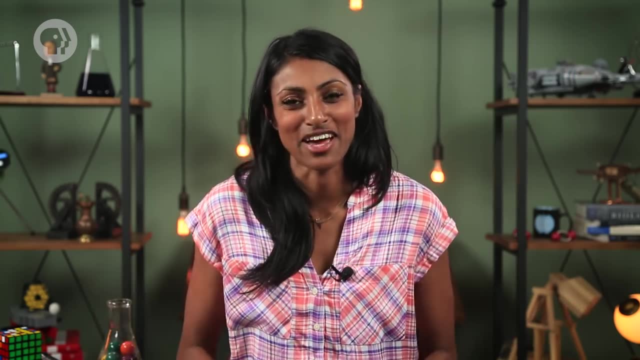 And this speed works out to be 3.00 times 10 to the 8th meters per second. We write it simply as small c, and it's the speed of every electromagnetic wave ever, at least in a vacuum. You may know it better as the speed of light. 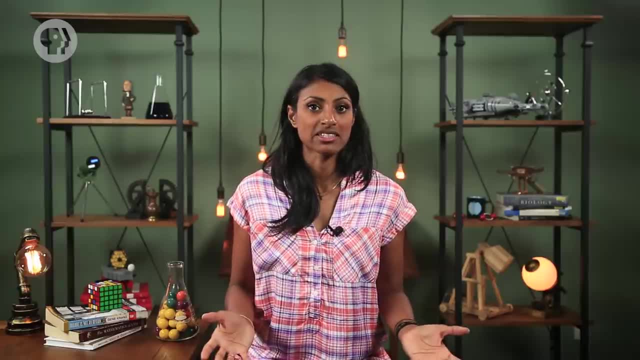 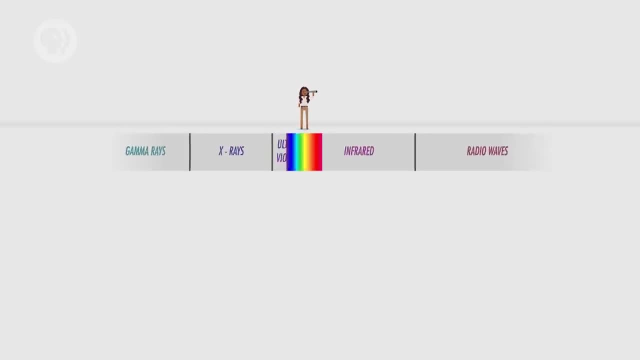 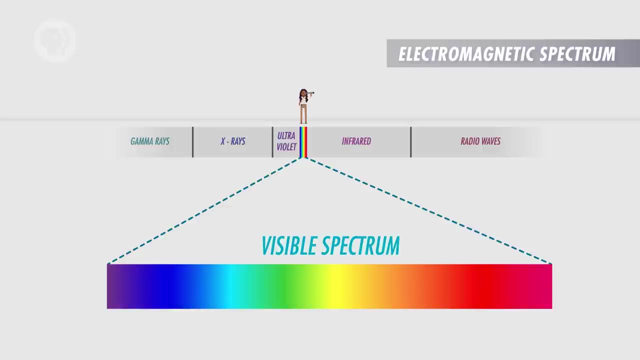 After all, light is an electromagnetic wave. Every electromagnetic wave carries energy through space and can reflect off some material while passing through others. Visible light is just one small part of what's known as the electromagnetic spectrum. Like waves in the ocean, electromagnetic waves can vary in their wavelength, amplitude and source. 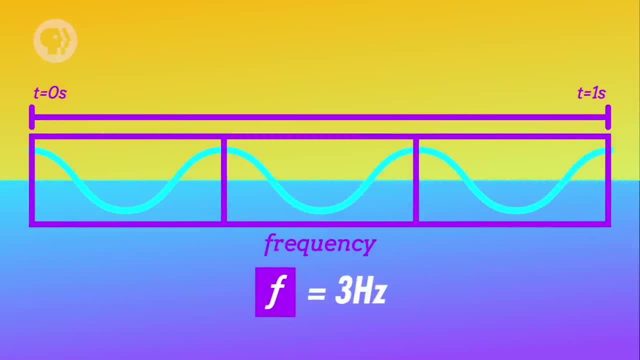 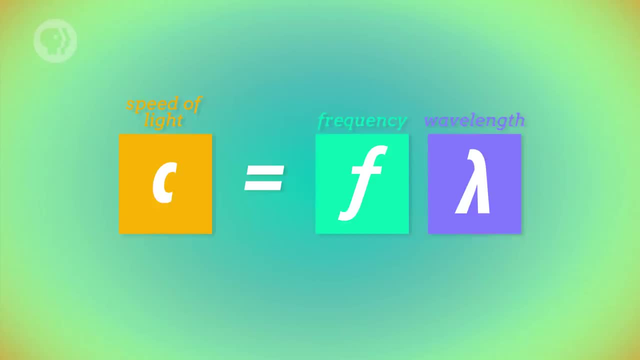 The wavelength is the distance between the peaks of the wave, and the frequency is how many times a wave peaks in a given second. You might remember, when we talked about travelling waves, that a wave's speed is equal to its frequency times its wavelength, And since the speed of light is constant, you can easily find the frequency if you know the wavelength, and vice versa. 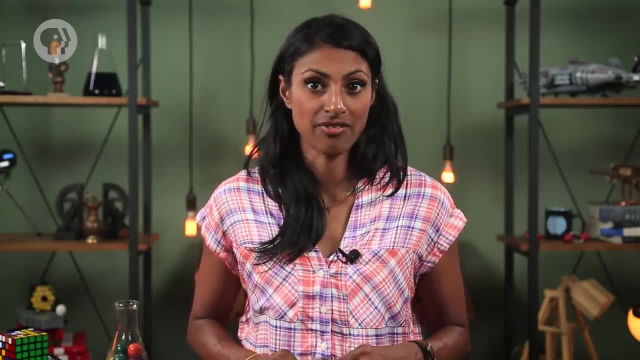 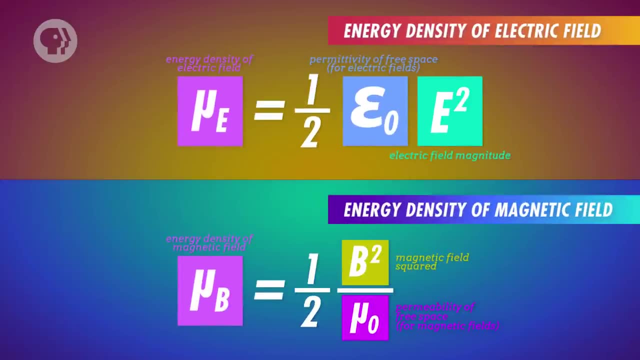 Now, in order to calculate the energy carried by any electromagnetic wave, you need to know the magnitude of the electric and magnetic fields that compose that wave. Specifically, you use these magnitudes to calculate what's known as the energy density of each field, which is the amount of energy stored in a field per unit volume. 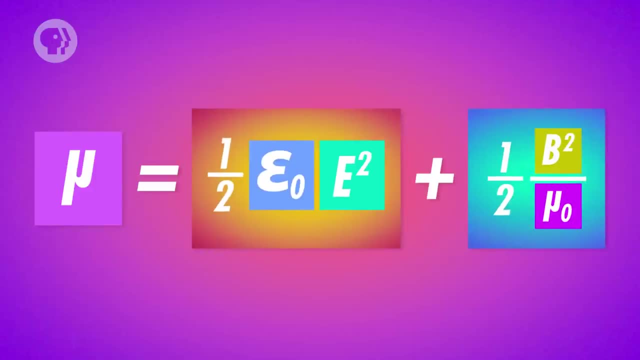 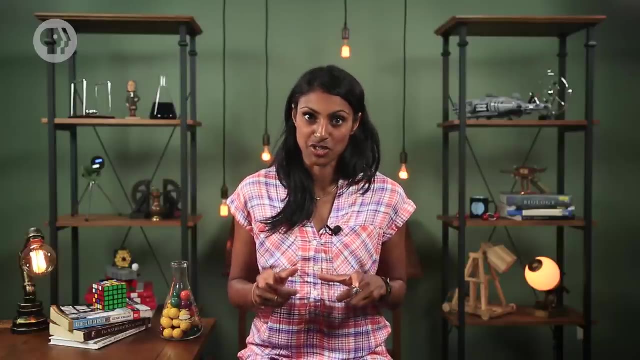 Then you can combine the energy density for both fields, solving for the total energy per unit volume within the wave overall. But since you know that the strengths of the electric and magnetic fields are directly related, you can substitute the electric field magnitude for the magnetic field magnitude. 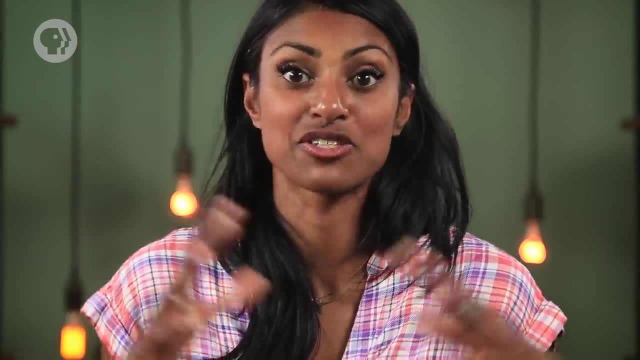 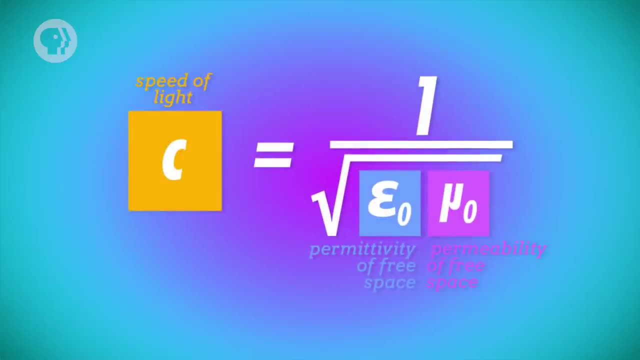 And vice versa. This lets you come up with the energy density terms that encapsulate the energy in both fields with fewer variables. So here's the calculation of the speed of light that Maxwell found and the constants that it's simplified down to. 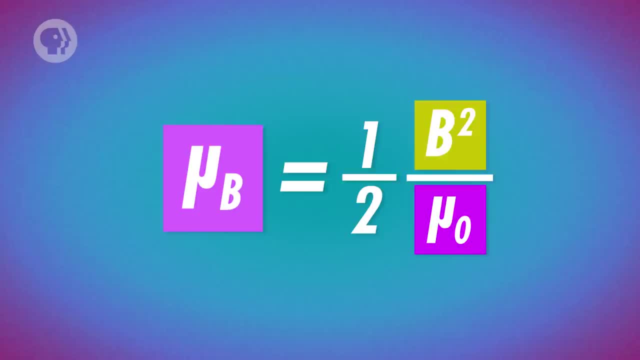 You can take our energy density equation and substitute the magnetic field magnitude B with the electric field times, the square root of the permittivity constants. With this simplified energy density equation you can then substitute the electric field magnitude for the speed of light and the magnetic field magnitude. 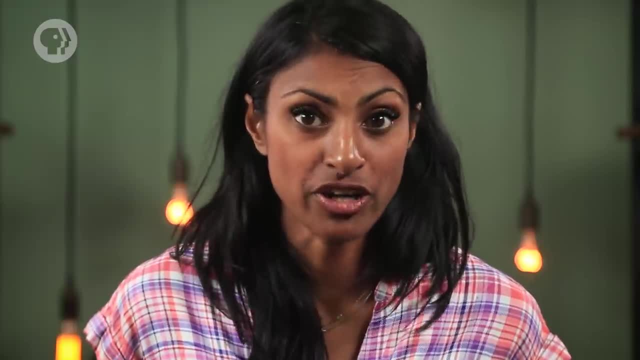 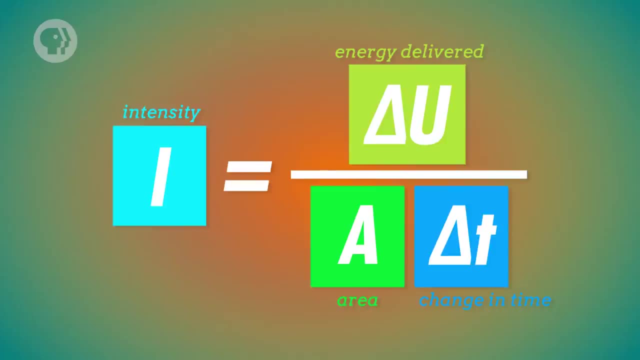 These equations give the energy density of an EM wave At any point during its propagation. One last important measurement of delivering energy is intensity, which is the energy transported by a wave per unit time, per unit area. Mathematically, the energy delivered, delta U is equal to the energy density times the volume of space in which the energy is transported over a period of time. 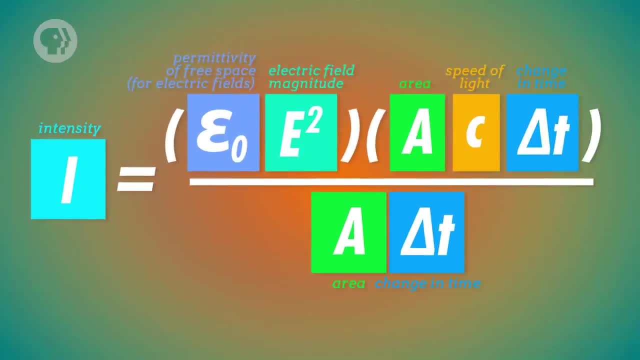 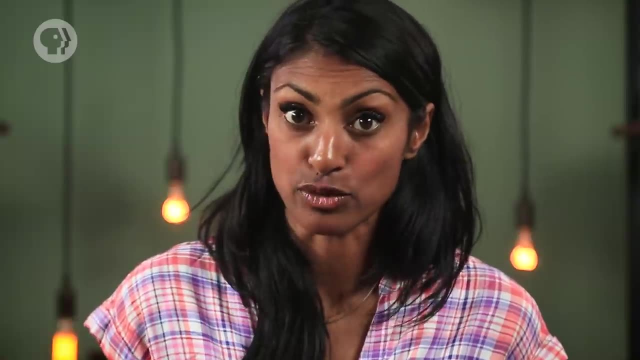 You can then replace energy density with one of the simplified equations we used earlier. So the volume of space encompassed by the wave is equal to the unit area times the distance travelled. And the distance travelled would be the speed of light multiplied by the distance travelled. 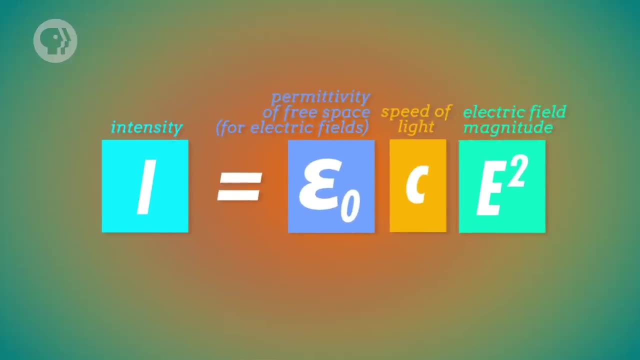 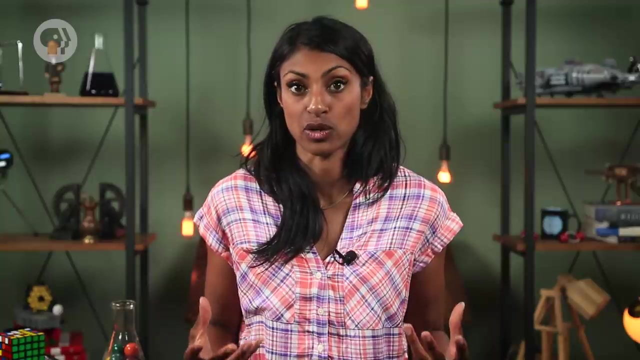 After cancelling out like terms, you're left with an equation that tells you how much energy you have per unit area, based on the strength of the electric field, which you can also replace with the magnetic field magnitude. A lot of math I know, but the vast knowledge of electromagnetism that we have today and the doors it has opened into the fields of relativity and quantum theory are all based on the theories that Maxwell and his predecessors developed.